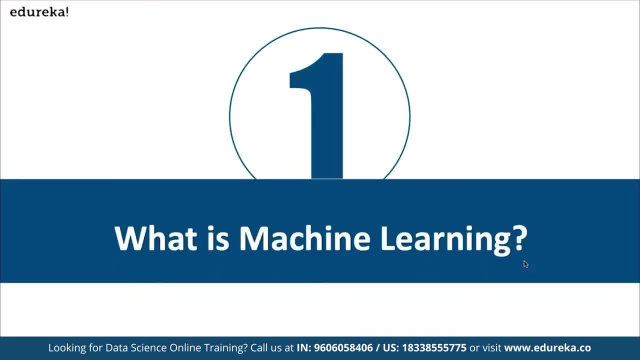 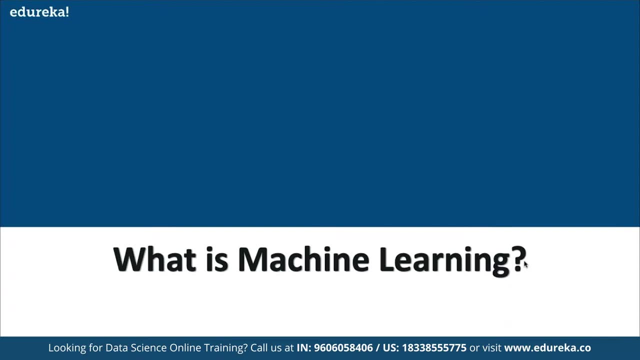 about machine learning itself. So what exactly is machine learning? So what exactly is machine learning? So machine learning is simply making sure that we are going to automate the entire system by using a good amount of data set. right, So we can say machine learning. 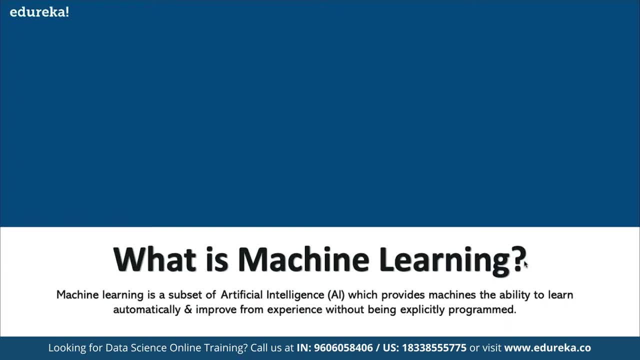 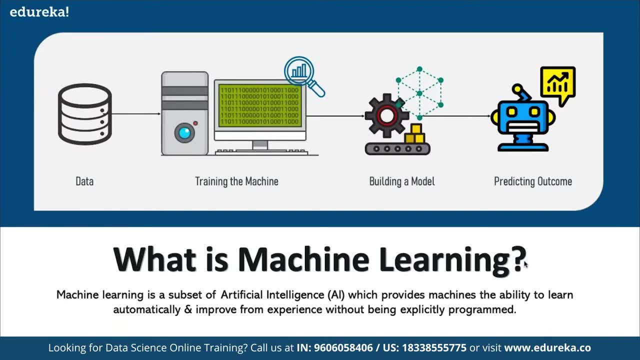 is simply the process of feeding a machine enough data to train and predict a possible outcome using the algorithms with which we have the access to. So, basically, if we use more data set, then we can increase the accuracy of the results. And let's say, you may have used multiple predictions made in support before any major match, right? 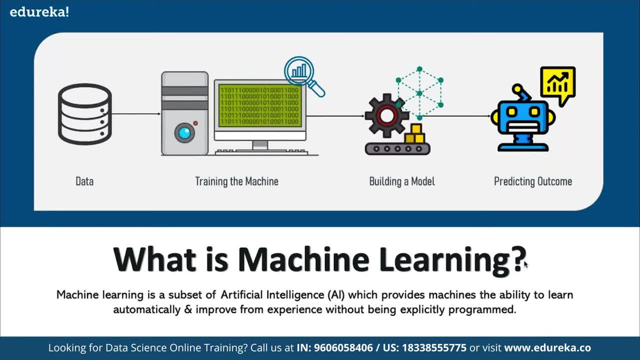 So in this case let's take an example for a football penalty session. So the data of previous performances are going to be considered. So let's say the goalkeeper has saved all the penalties to his right in the last 50 penalties he has saved. Now this data will. 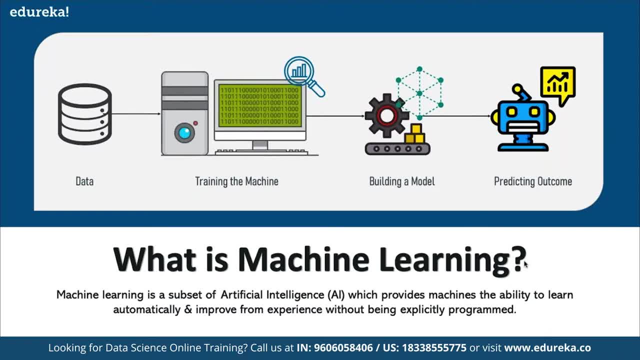 be crucial to predicting if he or will will save or he will not save the next penalty faces. So there are other factors to consider as well. Now, another example can be the suggestion that we get while surfing the internet. So the data of our previous choices are processed to give us the most favorable content. we are 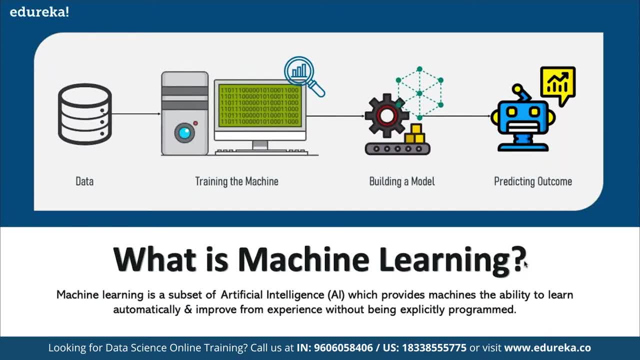 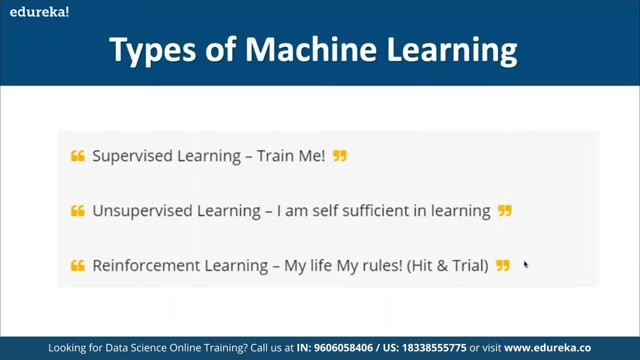 most likely to watch. Anyhow, machine learning is just feeding the machine an ample amount of data. There goes a lot of processes, algorithms and a set of factors to get the optimum results All right. So here, basically, we have three main types of machine learning as well where 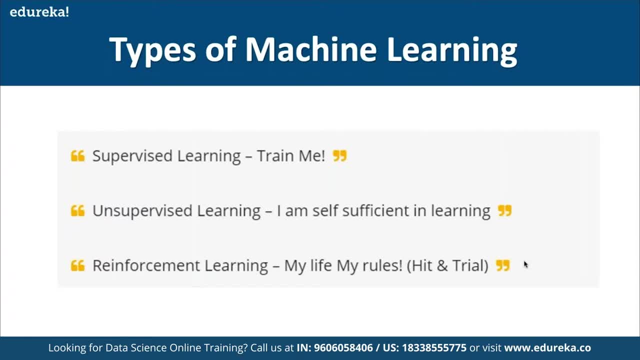 we have supervised, unsupervised, And then we have virtual And then we have reinforcement learning. So supervised in simple terms is: train me. It works on a simple training. We have to train the model, then only it can work. And an unsupervised learning is: I'm self-sufficient in learning based on their own learning. 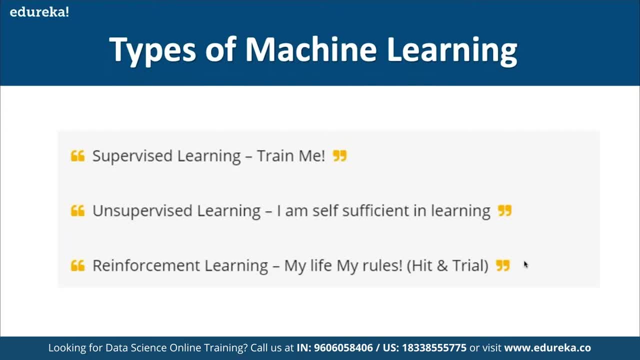 We are simply going to allow them to have again, to allow them to have the access as well. So that is what we are going to do. So, based on their own understanding, they are going to work accordingly. That's how it's going to work. 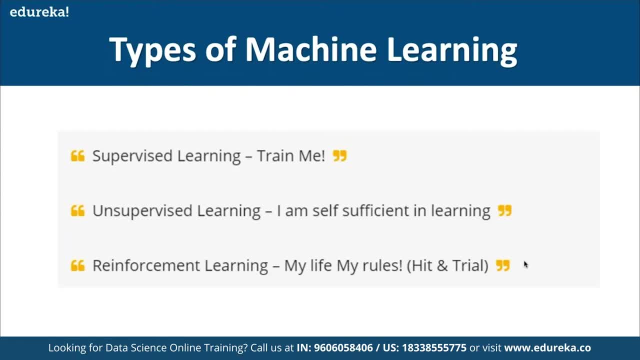 And then we are going to work on reinforcement learning. So reinforcement learning is simply learning on its own, based on the feedback we simply create. We simply let the system know if they have done a good job or not. based on that only, they simply try to get the best possible output. 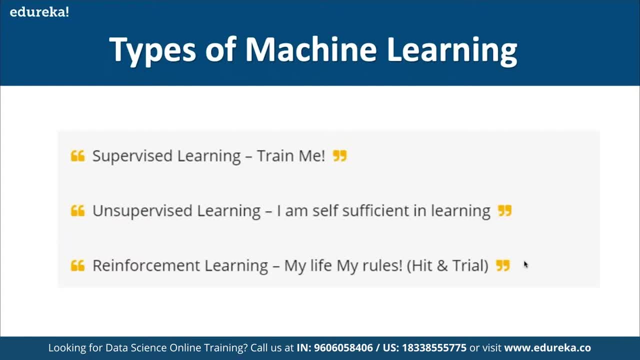 That's how it works, All right. So supervised learning: supervised learning, we use multiple label data set to train the system And under unsupervised learning, we use unlabeled data set. So the data is sometimes unlabeled, or we can say uncategorized, and the machine makes. 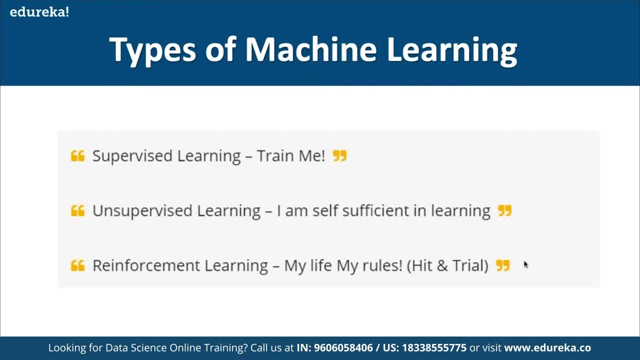 the best possible reference and predictions without any supervision. And then we have reinforcement learning. So reinforcement learning simply ensures that we are simply going to create a system based on the feedback. So the machine needs to establish a systematic pattern of approach in reinforcement learning. 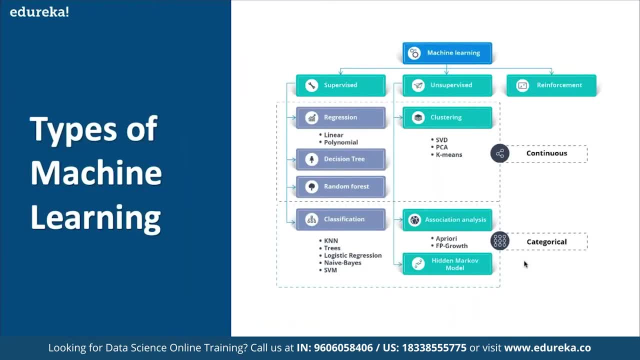 here. So that's how we discuss: Okay, Under unsupervised. again under supervised, we have multiple models, like we have regression decision tree, we have reinforcement models, we have different models currently available, Whereas in under unsupervised we have multiple models, like we have clustering, we have association. 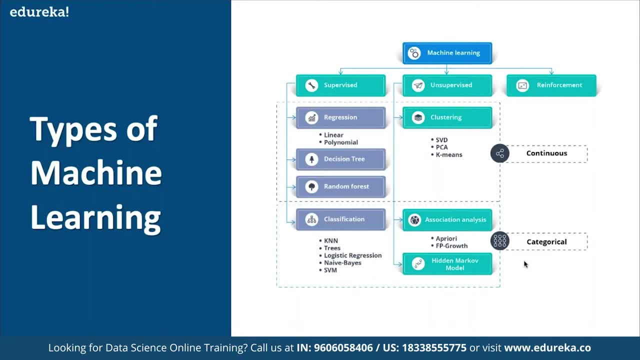 analysis, we have hidden Markov model. So again the KNN trees, logistic regression, Naive Bayes and SVM. they all are types of classification Where, if we talk about the a priori FV, growth K-means, PCA, SVD, they all are part of unsupervised. 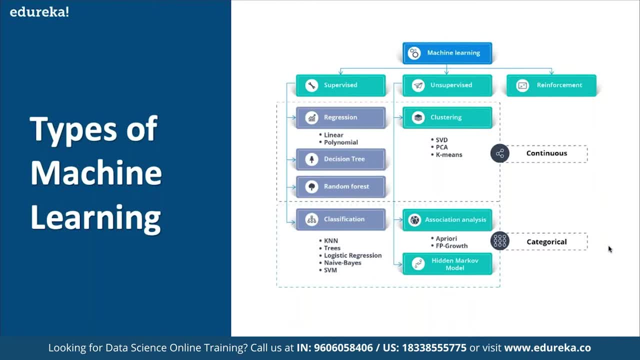 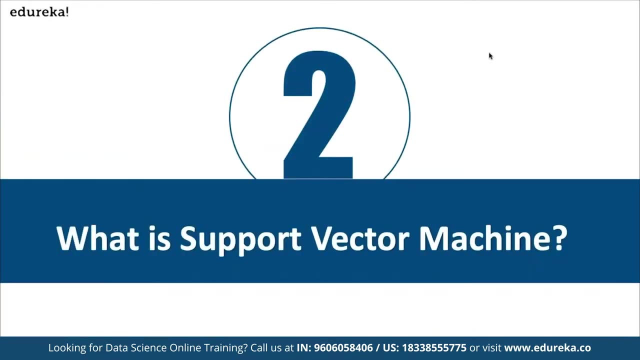 Okay, Under unsupervised. and again, reinforcement is simply based on its own structure that we are going to discuss as we proceed for the step-by-step. All right, So now, next is we are going to discuss on what exactly we mean by support vector machine. 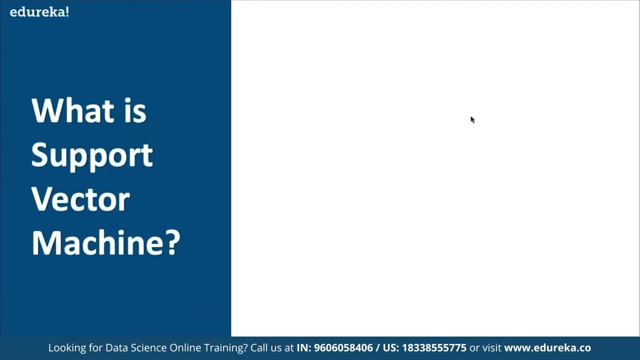 So a support vector machine was first introduced in the 1960s and later improvised in 1990s as well, And it is basically a supervised learning machine Classification Algorithm that has become extremely popular nowadays because of its, you can say, efficient. 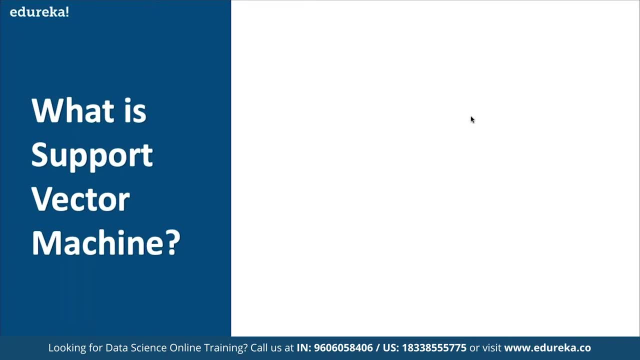 results and especially for the complicated scenarios, it can deliver it for us as a part of support vector machine. As you can see- I can simply- it is like a discriminative classifier that is formally designed by a separative hyperplane itself, And SVM is implemented in a slightly different way than the other machine learning algorithms. 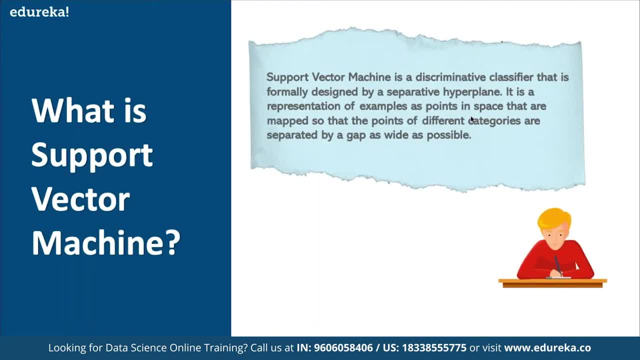 So It is basically a model of performing classification, regression and outlier direction as well, And support vector machine is basically again simply designed by as a separative hyperplane set, as we discussed. So basically here we can have multiple data pointers that can be mapped so that the points 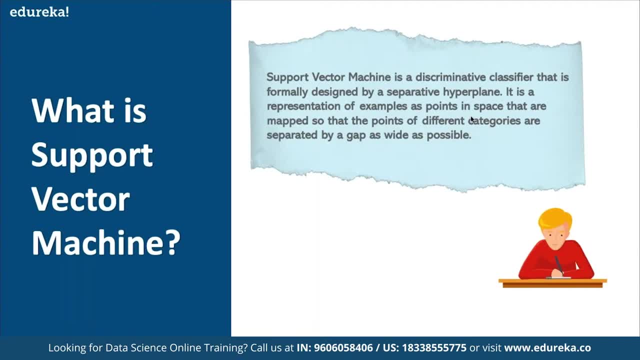 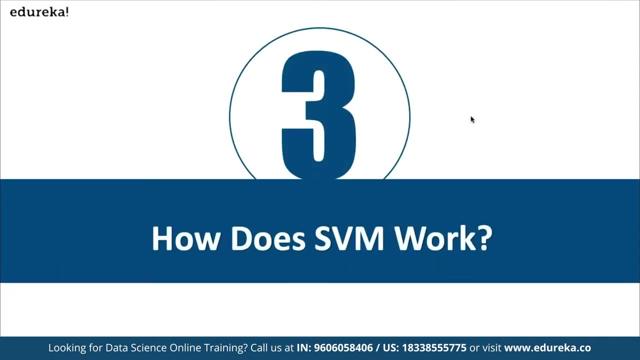 of different categories are going to be separated by a gap, And in addition. so basically SVM can also perform non-linear classification. So we'll be talking more about the How exactly support vector machine works as we proceed further. but there are multiple advantages of using SVM as well. 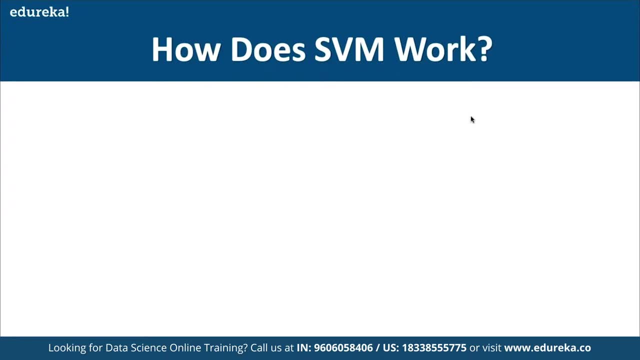 For example, it is effective in high dimensional spaces. It is effective in cases where the number of dimensions in greater is greater than the number of samples, And it is again. it simply uses a subset of trading points and decision function. that makes it memory efficient and it has different kernel functions that can be specified for. 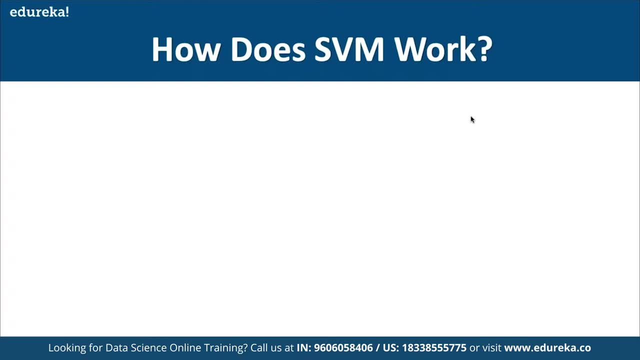 decision function. That also makes it And same way. we also have multiple, we can say downside or we can say disadvantages of using SVM as well, So the number of features is much larger than the number of samples. Then we can simply avoid overfitting and choosing kernel functions. 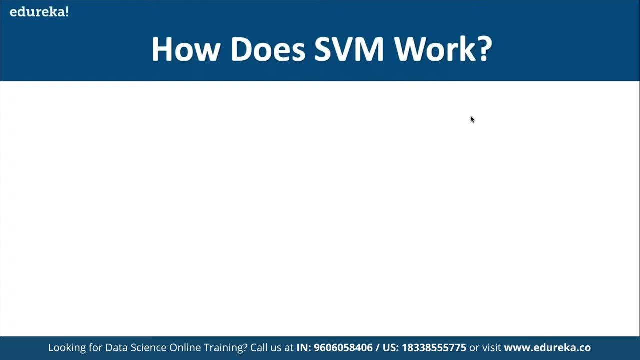 And again, recognizing them is crucial. and SVM did not directly provide probability estimates, And these are calculated using the five fold cross validation. And how does SVM work? So the main objective of a support vector machine is to segregate their given data in the best possible way. 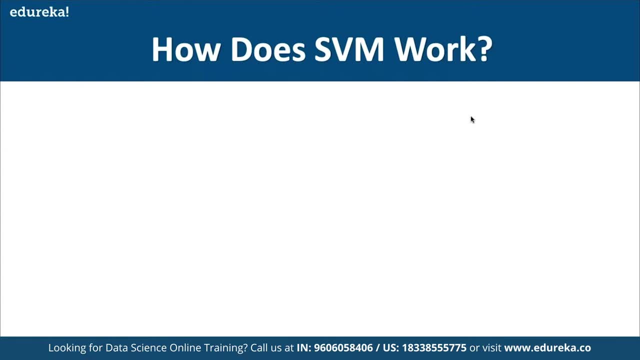 And when the segregation is done, the distance between nearest point is known as the margin, And the approach is set to a hyper- basically hyper- plane with the maximum possible margin in the support vector, As we can see here. that has been right now presented. all right. 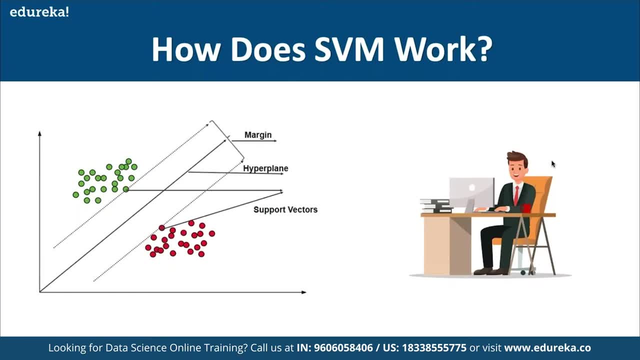 And now basically here to select the maximum hyper plane. So now here, in the given data. Okay, So in the given sets. the support vector machine follows again multiple sets, for example, is simply going to generate the hyper plane which segregates the class of classes in the 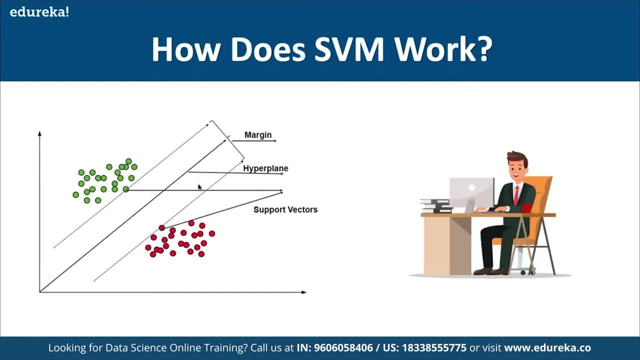 best possible way, And then we are going to select the right hyper plane with the maximum segregation from either nearest data pointers. So, basically, there are different ways of or even on dealing with inseparable or, we can say, non-linear planes as well. 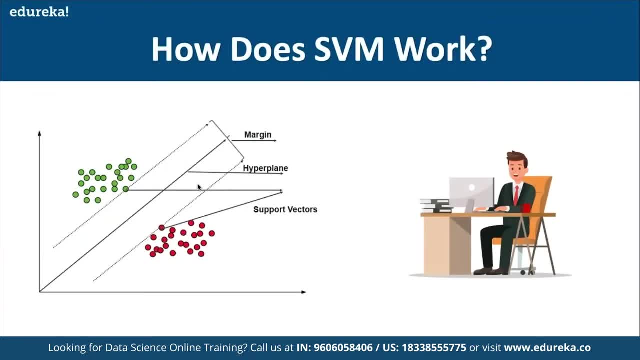 So, for example, in some cases hyper planes can not be very efficient, And in those cases the support vector machine uses a kernel tick, a kernel trick, to transform the input into a higher dimensional space, And with this it becomes easier to segregate the pointers. 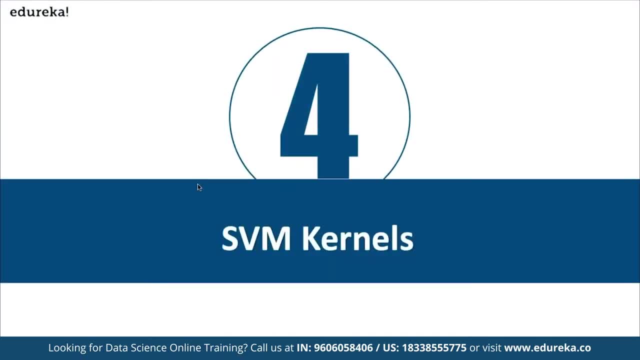 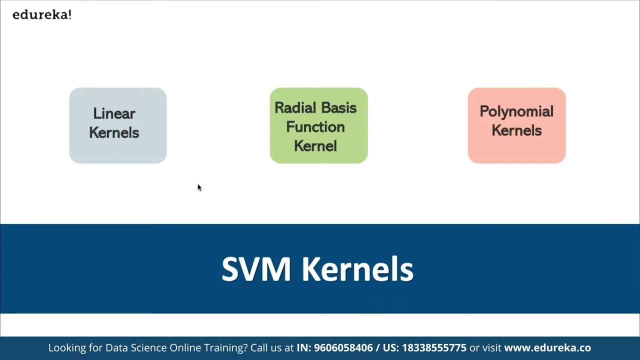 So now let's talk about the SVM kernels. So basically, SVM kernel adds more dimension to a lower dimensional space to make it easier to segregate the data. It converts the inseparable problem to separable problems by adding more dimensions Using the kernel trick, and a support vector machine is implemented in practice by a kernel. 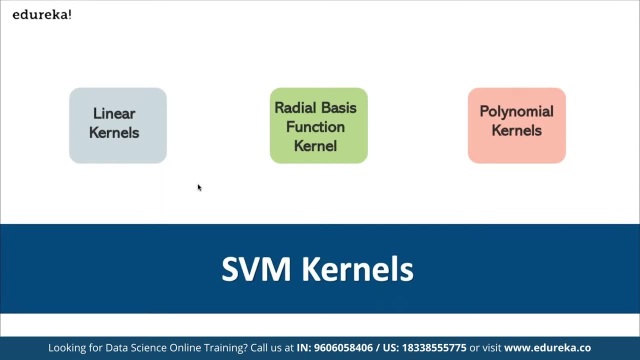 and the kernel trick helps to make more accurate classifier. So we can take a look at different kernels in a support vector machine, Like we have linear, we have radial base and then we have polynomial kernels as well. First of all, let's talk about the linear kernels. 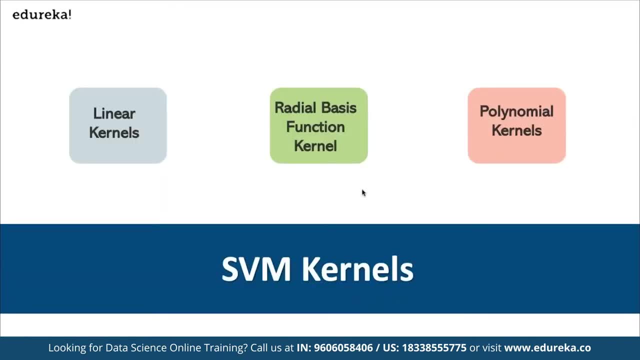 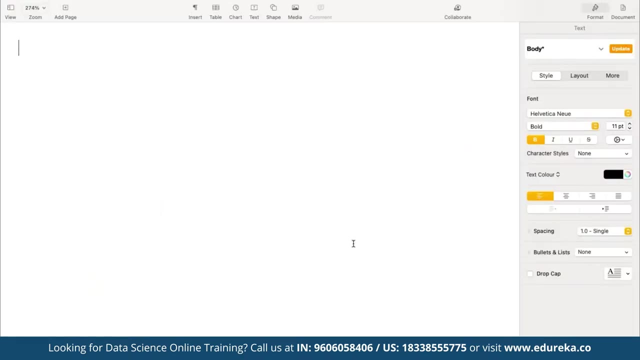 So a linear kernel can be used to as a normal dot product between any two given observations. So the product between the two vectors is the sum of multiplication of each pair of input values. So we can understand this. So if we talk about the linear kernel, 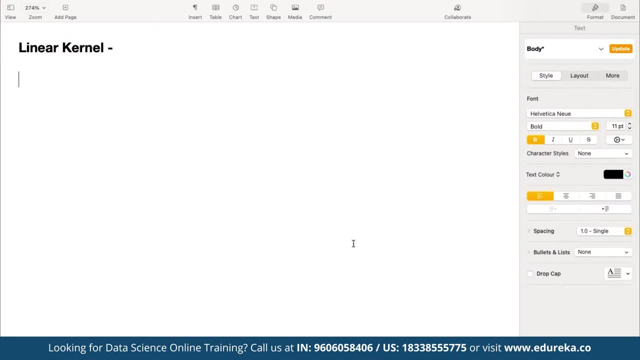 So basically, as we discussed, linear kernel can be used as normal dot product between any two given observations. For example, here we can find this one as opposed to zero, and it can be added to some observations. So this is the sum of, let's suppose, multiplied by X, X. 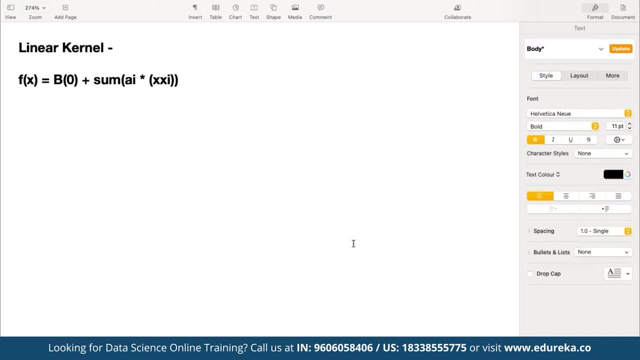 All right. So, as we discussed again here, it is going to be the product between two vectors and the sum of multiplication of each pair of input values as a part of simple linear kernel equation, And then we have polynomial. So this one is for linear. 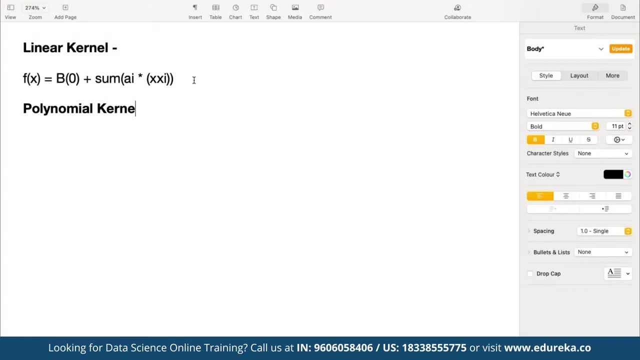 Then we have for polynomial kernel. So polynomial kernel is for. polynomial kernel is like a it's rather generalized form of the linear kernel, And again it can distinguish curve or nonlinear input space. So for example, here we can refer this as opposed as K, and then we can define multiple. 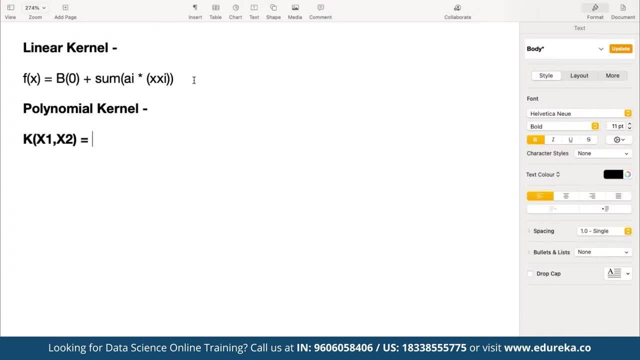 pointers, I suppose X1, X2.. And then we can simply add this to a plus. Now here we have to find, suppose X1,, and again all of that could be defined here: X1, T and then X1.. 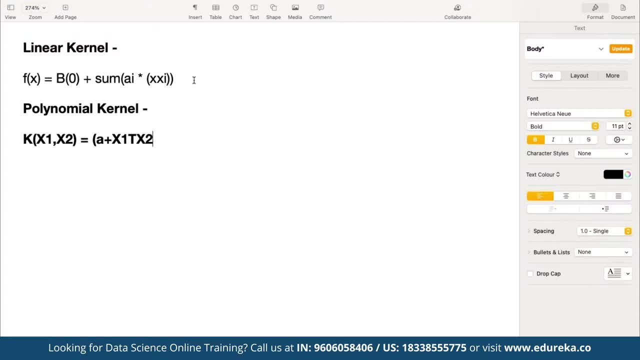 So this could be, let say, for one of the two groups. Okay, Cool, Un понад terms of radial basis function kernel. so here the radial basis function kernel is commonly used in the svm classification and it can map the space in infinite dimensions. so basically, if we talk, 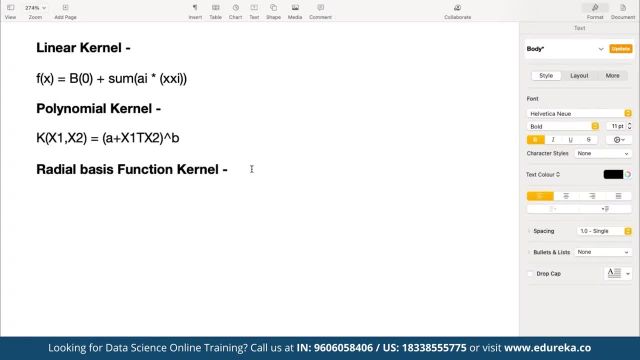 about the actual dimensions here. so here we can represent it as suppose the value of k, x1, and again for x2, and here we can find the exponent where expert is going to be supposed for minus 4, again the gamma value, and let's say we represent this as y, and then we can define this for. 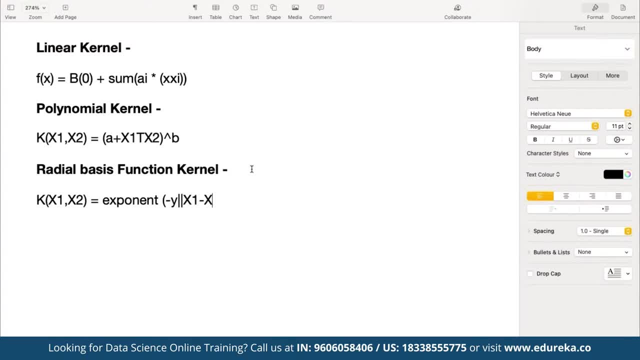 x1 minus this is going to be x2, and then it has to be raised to power 2.. so basically, x1 minus x2 is simply going to be the euclidean distance between the x1 and x2, so we can say x1. 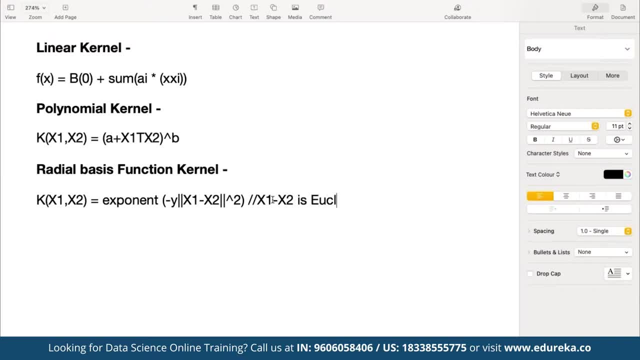 minus x2 is euclidean distance, is the euclidean distance between x1 and x2, here and where, if we talk about here, if we talk about the current component for b. so here we can say: b is what b is, b is the degree of kernel. in case you don't have, we can, in case you don't have the knowledge of: 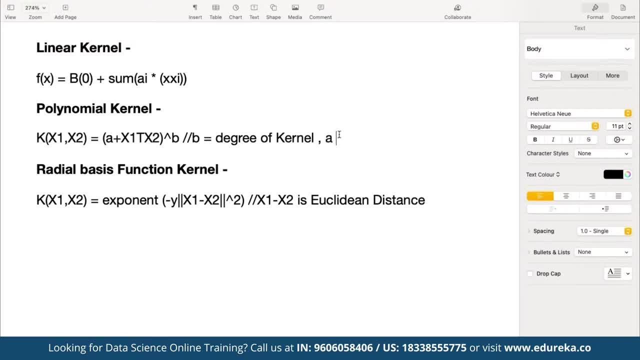 operative and then a is going to be. or you can say: a is what, a is the constant term is the constant term that we have. so here we have linear polynomial and then we have radial basis function, so there are multiple use cases. so, before we proceed further, so there, 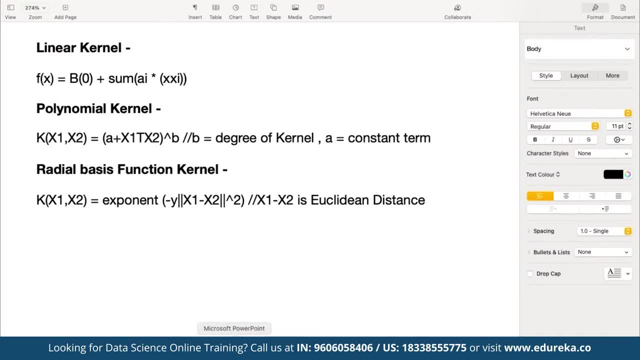 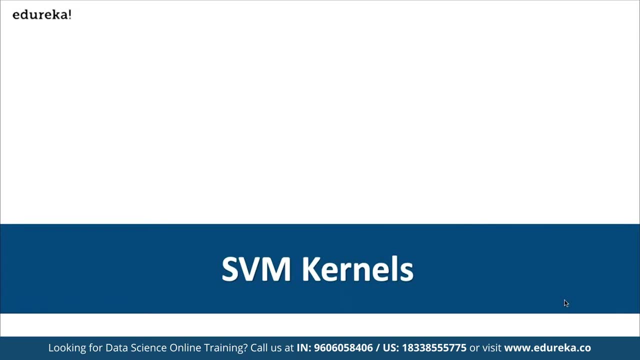 are multiple use cases of the serial base conver- i can say component as well. so here we can use it for the phase selection, for text and hypertext characterization. here we use it for the classification of images, for bioinformatics, for protein fold and remote homology detection as well. 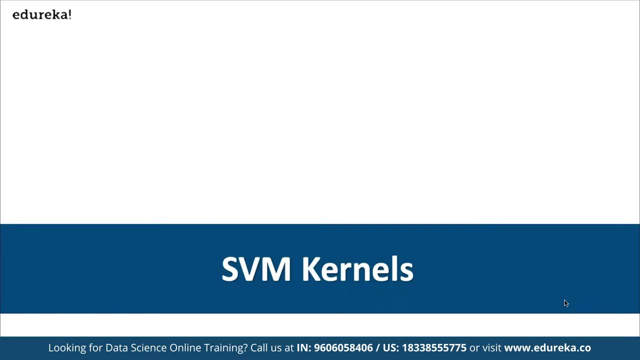 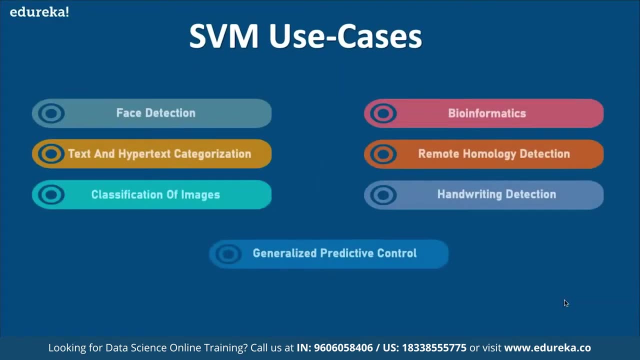 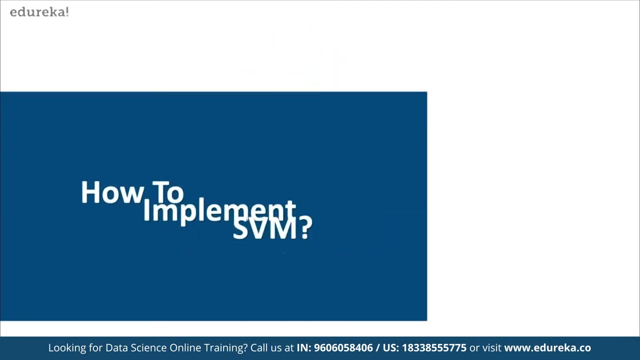 we can use it for different use cases and we can also use for, again, having a prediction control as well, as we discuss in svm. so there are multiple use cases for phase selection, for bioinformatics, for text and hypertext categorization, for remote homology. so these are different use cases are currently available here. so now, in terms of how to implement, 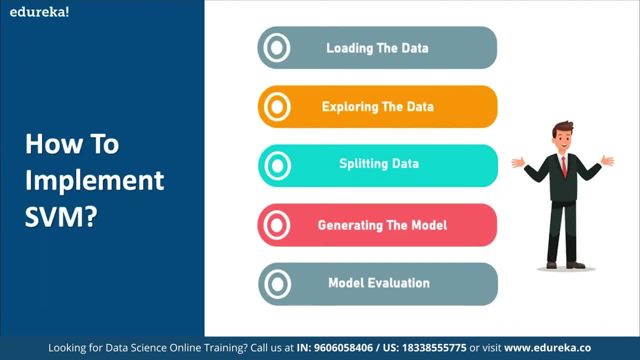 svm. so first of all, we have to load the data, we have to explore the data, we have to split the data, and then we also have to generate the model and then we have to evaluate the model as well, as we have discussed again in case we have been confused. so linear is simply going to 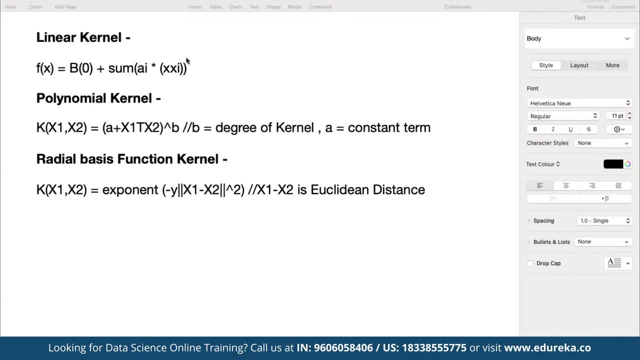 be the dot product between the any two given observations itself. and here we define two. uh, here the pro is going to be between two different vectors, it's simply going to be the sum of multiplication of each pair, and then under polynomial. so basically here we can distinguish curved or non-linear input. 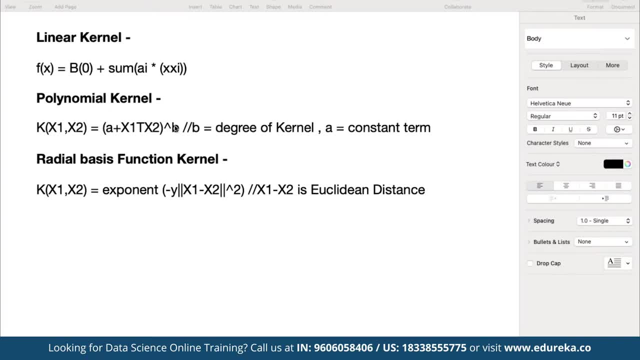 space where we have defined the k1 as x1, x2 for where a is where a is simply going to be a constant term and b the power to which we have increases. so b is simply going to be the degree of penalty we are going to make use of and then, under radial basis, as we discussed, it is. 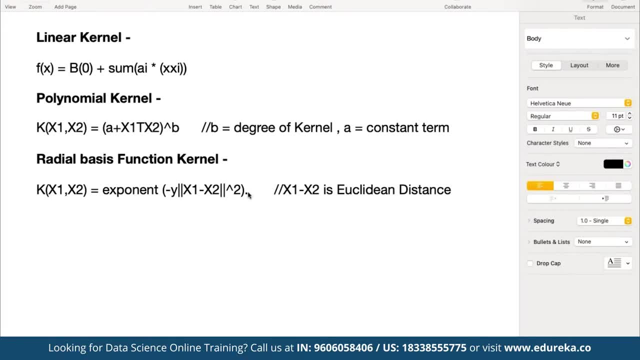 commonly used in classification and can map the space in infinite dimensions as well, where x1 minus x2 is simply going to be the euclidean distance. and we can say this one that we define here, x1 minus x2 here is simply going to be the euclidean distance here. all right, so 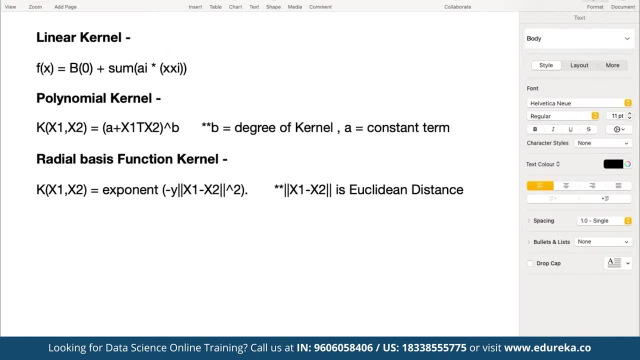 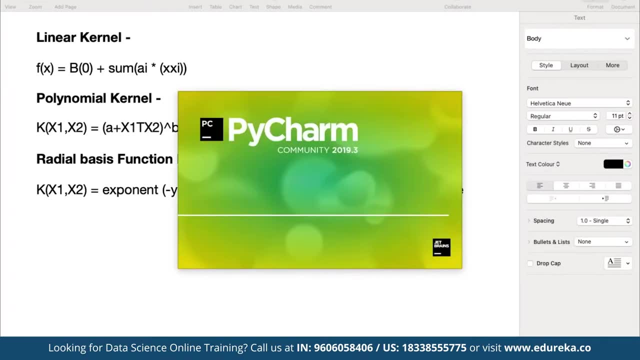 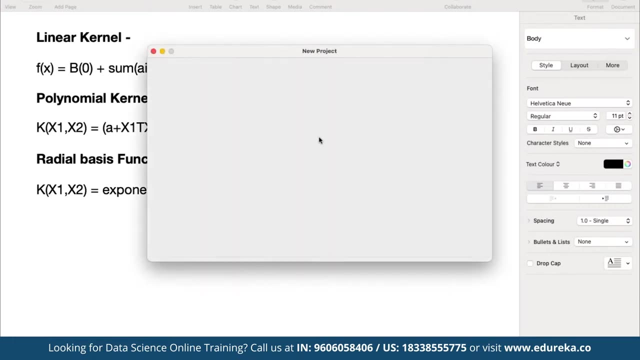 let's do one thing. let's open up pycharm community here so we can start by simply loading the data set and then working on top of it. so we can use any id. we can use any python id to get started. we can use anything. so let's do one thing. let's create a new. 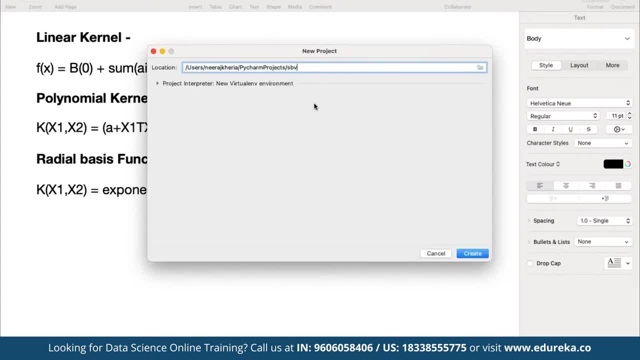 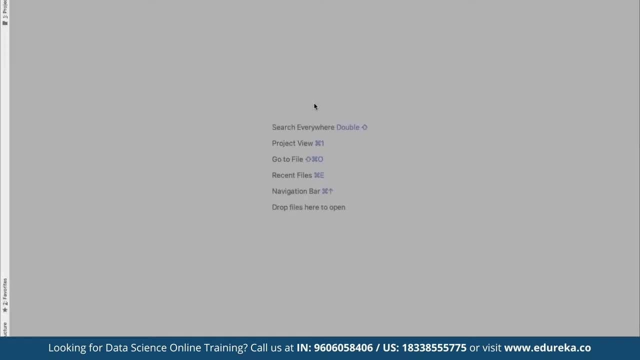 project. let's say we name it as svm. so in case you don't have the access to svm as of now, so you can go ahead and download the community version. so this is going to give you the access to pycharm, or we can use any other id as well if required. all right, so here, once we end the project, here we can. 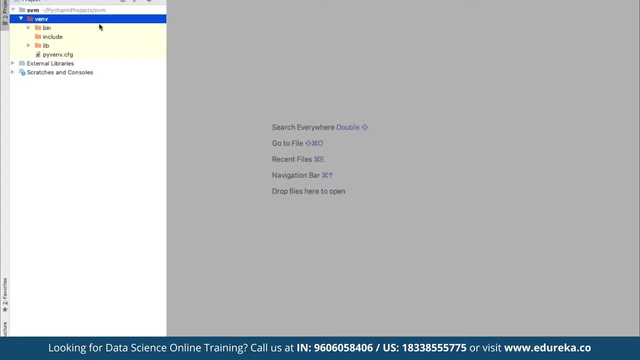 go ahead and create a new file altogether, so let's name it as our demo file. so first of all, we are going to work from the skln library, so here we can use from skln. we are going to import the data set, so they they are some sample data set available under 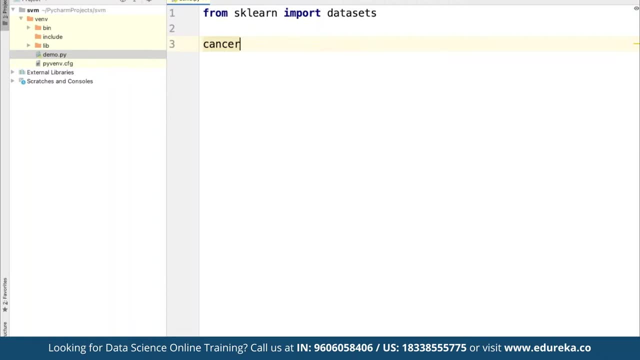 skln library itself. so here we can define the cancer data set already available under skln, and here we can use data sets dot load and then we are simply going to load. suppose, for breast cancer we can load this current data set already available. and now, if we want to simply print the 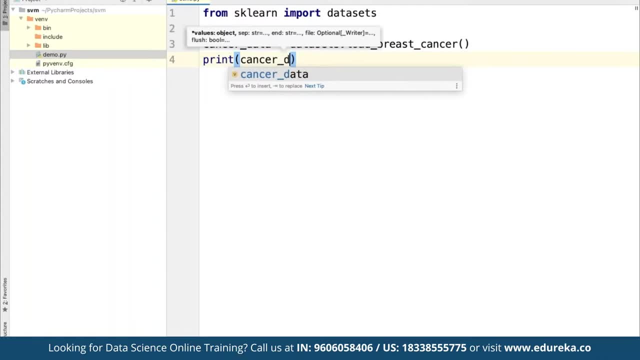 current data set that we can, that we have currently imported. so here we can find cancer data, dot data and again we only want to print the five first rows available in that. so here we can define these statements here. so we have- we are going to use a sample data set currently. 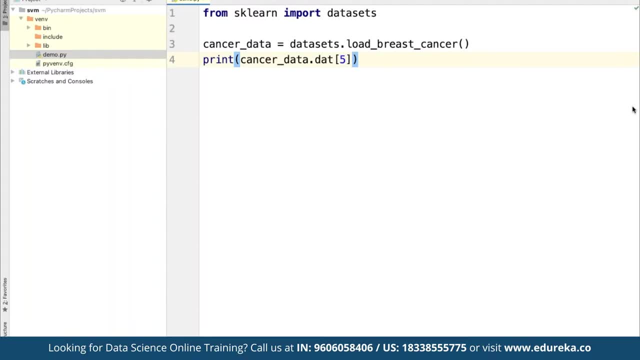 and whenever we are going to work on any project. in case they are now, in case the data set is not available, then we can go ahead and simply install more libraries by simply choosing the current data set, and then here we can go ahead and click on add and from here we can search for any library. 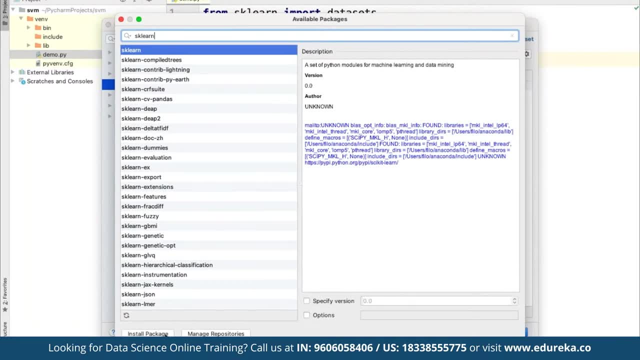 that is, that we may that may be missing. for example, here we are going to work on sklan, so we have to make sure that we do import skl, because without skl library we will not be able to work on the spm here. so here we are simply going to work on the sample data set. 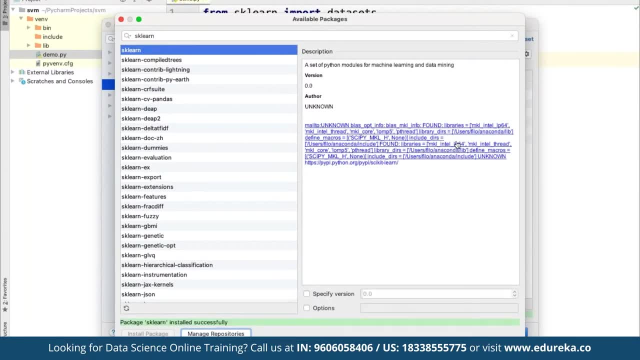 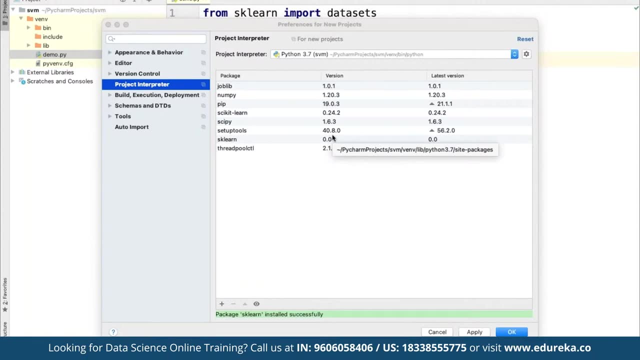 all right. so, as you can see, now skln has been installed. so again, this is a, this is a packet that we're going to work with, so here we can close it. if we want to work on the other components, we can search for any library and then we can have it installed. all right, so 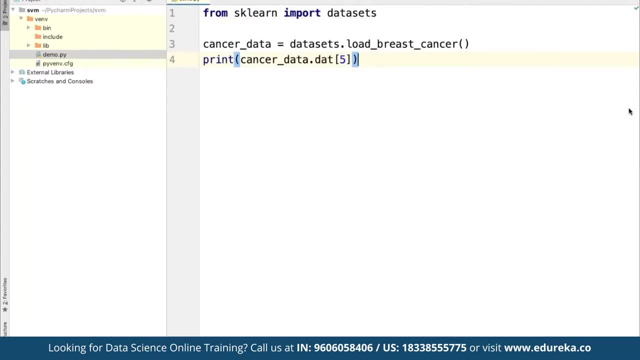 now we can click on apply and then, once we now, because if, if we don't have the library installed, and then if we try to run this up, it will simply go to throw us an error and, as you can see, currently this is going to update the package and then from there it is simply going to 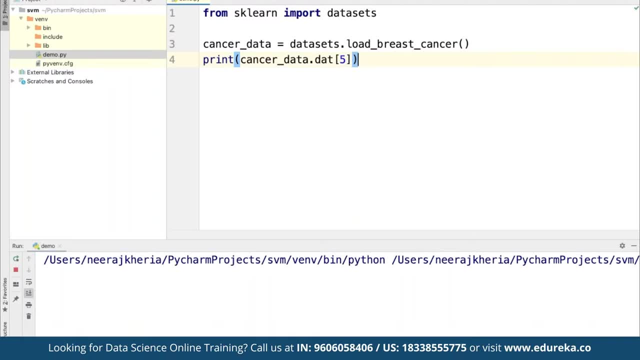 load the breast cancer data set, which is available as an inbuilt sample in sklan. so it is simply going to get connected to the server and then from there it is going to be going to pull the load- the breast cancer leader set- and then it will simply go to print the first five rows from that data set. 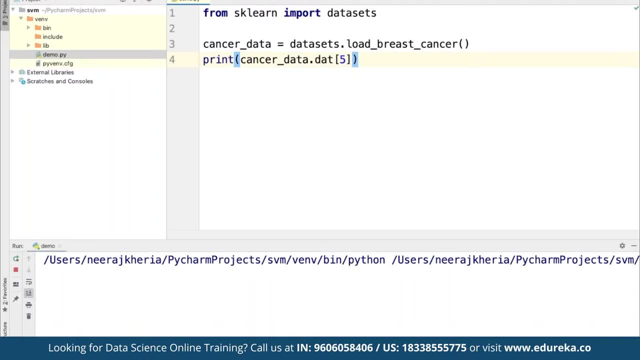 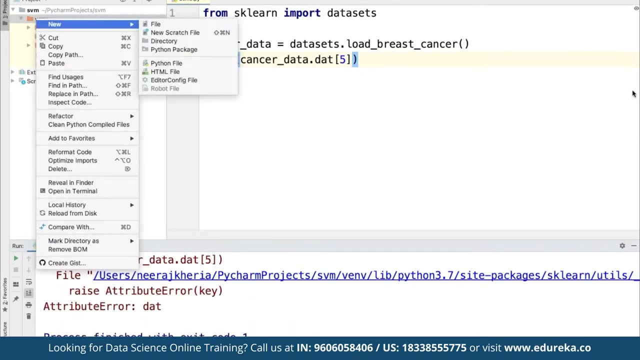 as well, depending upon how which data set we have imported. so before we perform any calculation, let me just show you how certainly this looks like. again, in the meantime, this is getting pulled here, so we can simply go ahead and create a new file. it has been timed out because of memory error. 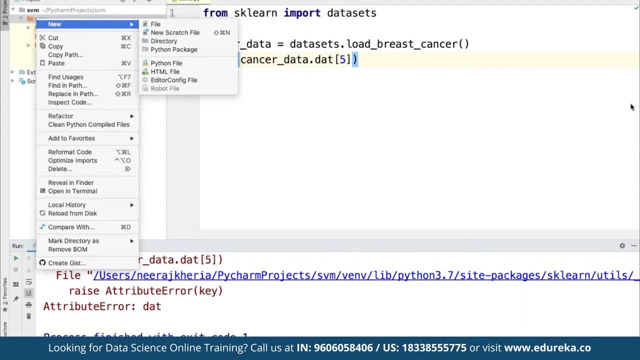 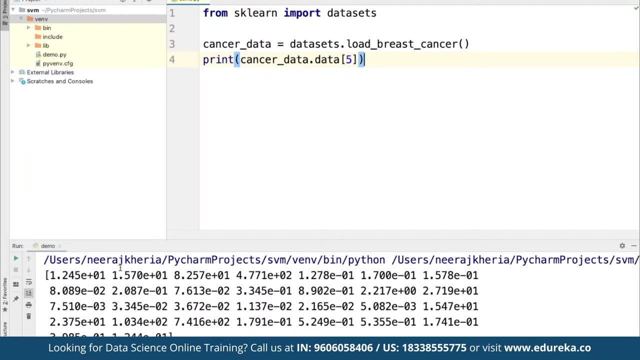 okay, we defined, we misspelled data. it has to be data itself, that only december going to data from there. so, as you can see here, now we have the first five rows in terms of this press cancer data which has been pulled automatically from sk none, as you can see here, right, so now, 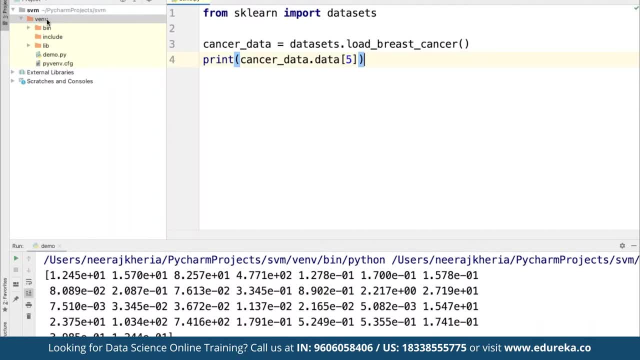 we are going to here. we have defined the data set right, so now, if we are going to simply split the data, right, so we are simply going to divide the data into trading set and the test set to get accurate results, and after this we will split the data using the train. 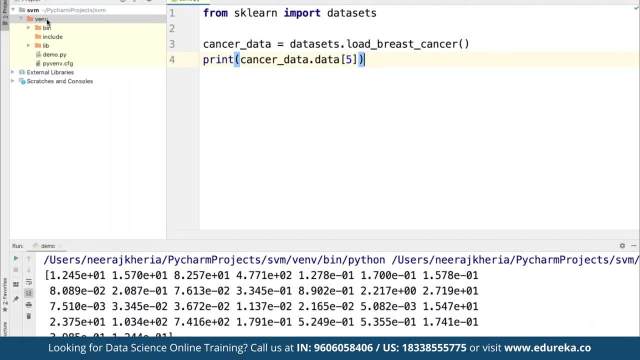 test split function. so here we are going to need three parameters, like in the sample that we have, that we are going to see. so from here we are going to load the current data set. so, for example, now here, now, just to avoid confusion for you all, so we can create a new. 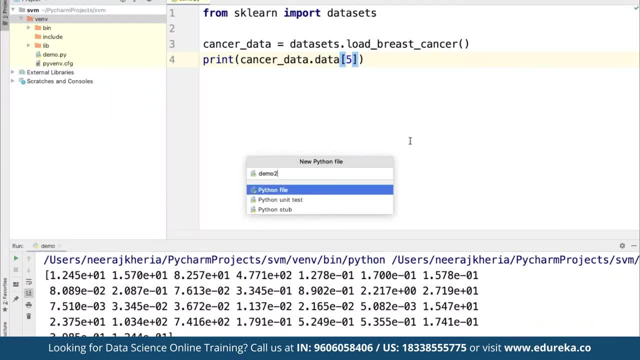 file. let's say we define some as, suppose, number two. so here we can define from sklearn. so first of all we define from sklearn library, from sklearn product dot model, and here we can define model selection. so here we are going to import train test split, as we discussed, we are going to spread it and then we can define from cancer. 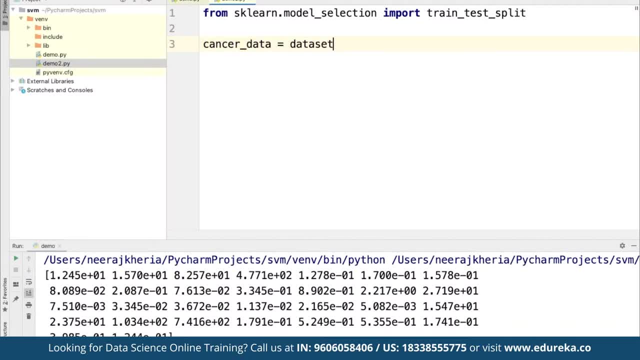 data that we are going to import. so here we are going to find data set, dot load, rest cancer, which is already available, and then we are simply going to define model selection and we can create a model with a model build model model. We need to think of this from a model. 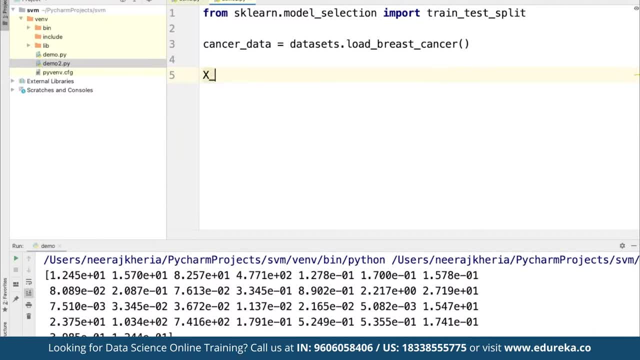 model. that is already here and we need to define 구조�ffmode by del and to the model, the models, in terms of: suppose here we define x train and then we can define x split. we can define for x test and then we can define same thing for y train, for y test, x train. 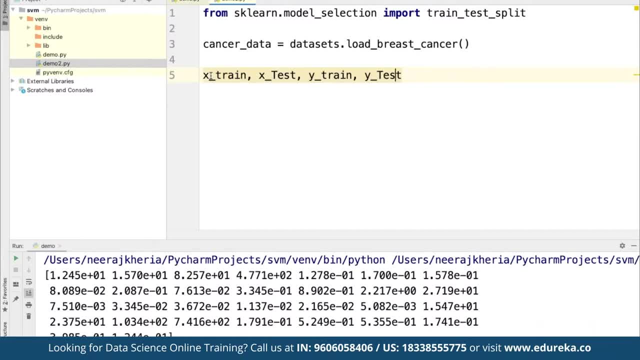 x test, y train y test. so here we are going to define this from the same train test split that we are going to import, and then here we are going to divide them under from the cancer data and the data which has been imported here, and then we are going to define this for cancer data target. 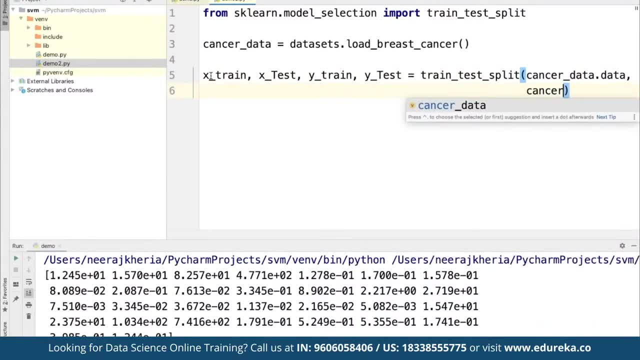 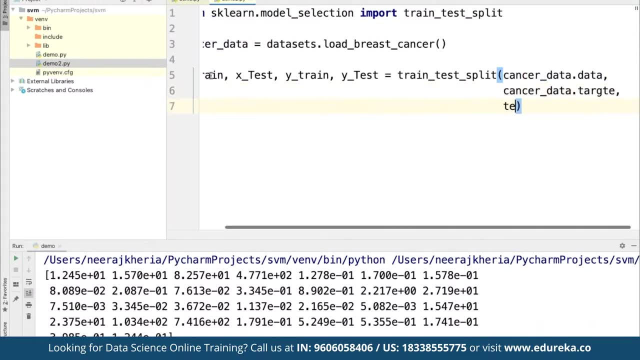 so say, here we can define this for cancer data dot target. and then we can define the test size. here we can define the test size. suppose we want to keep the test size, suppose as four, let's test such as four, and then we're going to find random state. we're going to find random state. 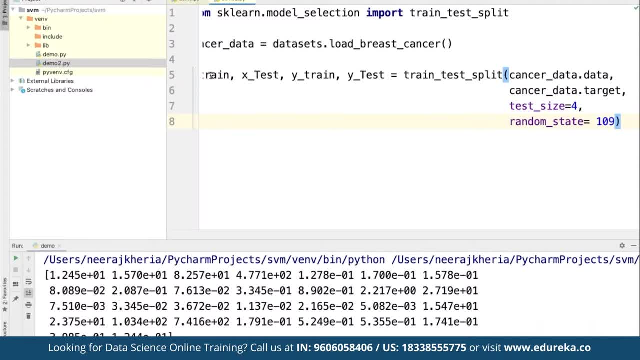 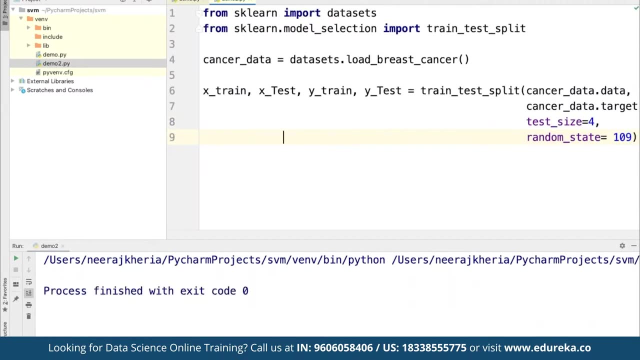 and suppose we don't like anything that we want to have. so here we are simply going to split the data set with the given in the x train, x or x test and the y train and y test here. so here the entire set is simply going to be split. so, as you can see, now that we have split, 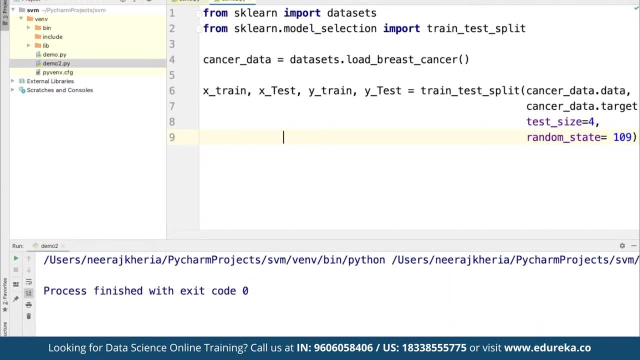 the entire data set. so now we are going to generate the model as well. so what we can do. so now, here we are going to gen. we can say: generate the bottle and for that we can import, on the library, for example. here we can import, let's say, sk learn. 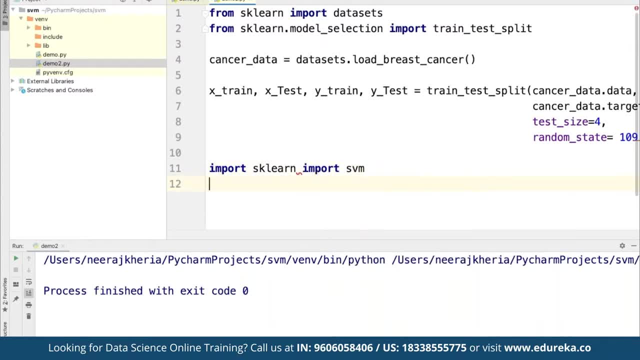 and here from sql we are going to import the svm. so here we are going to create the library. so here we could create a classifier here. so first of all we're going to find classifier as opposed svm, dot, svc, and here we're going to find the kernel, here we can find the kernel. 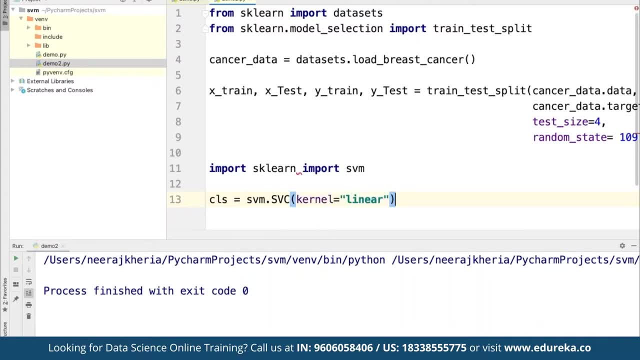 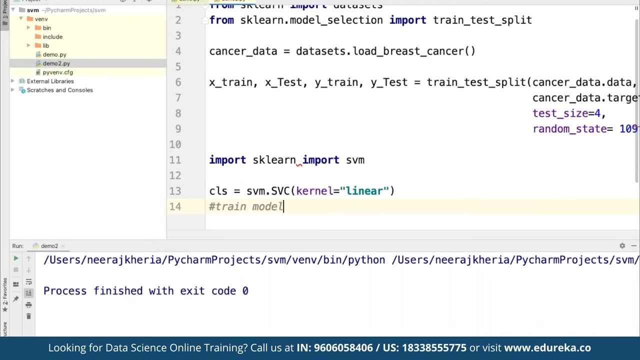 as opposed at, also as opposed linear, whatever we want to use. we can define that and then we are going to train the model. so we can say we are simply going to now train model. so here we have create classifier and now we are going to train the model. so 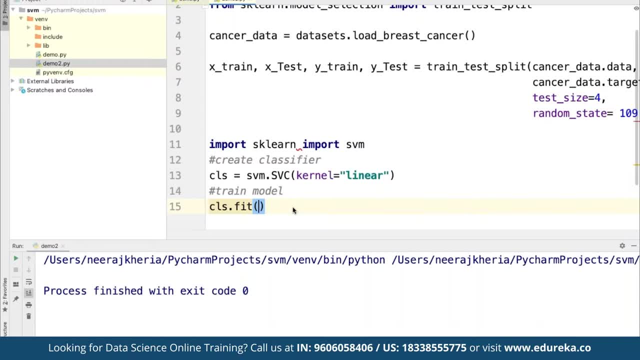 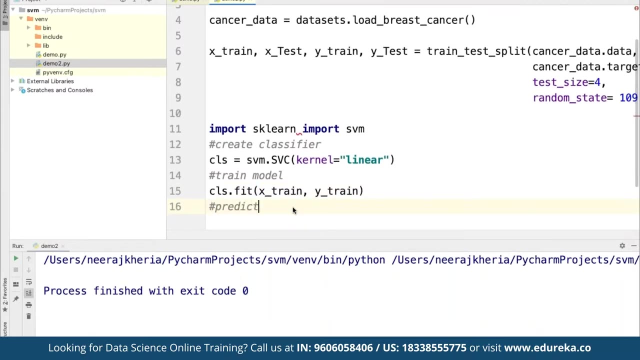 for training one. we can define class, dot, fit, and then we can define this value as extreme that we have already imported and then we can define for white rate that have we have already the split on and then simply we are going to have a prediction done. so here we can define predict. 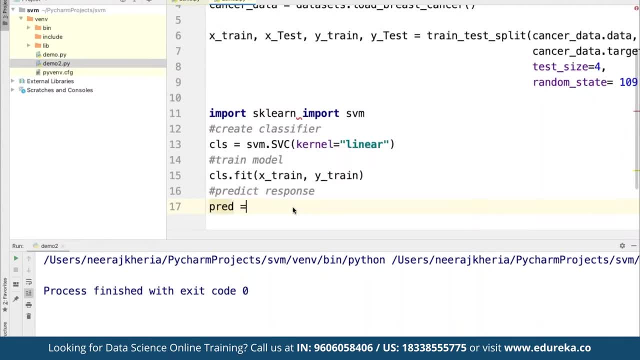 response and for getting the response. we can define prediction as class dot predict, and for this we are going to make use of x test that we have already defined. we have defined for x train and for y train, and then for prediction we are simply going to do that on the 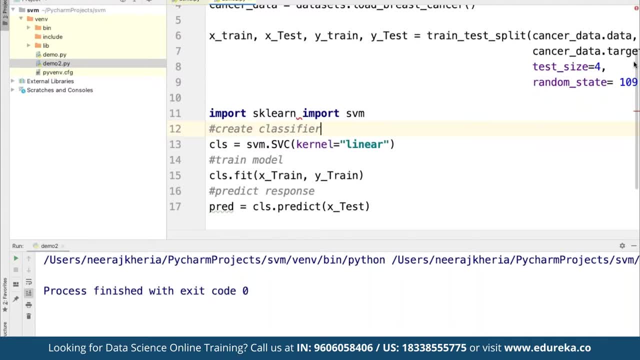 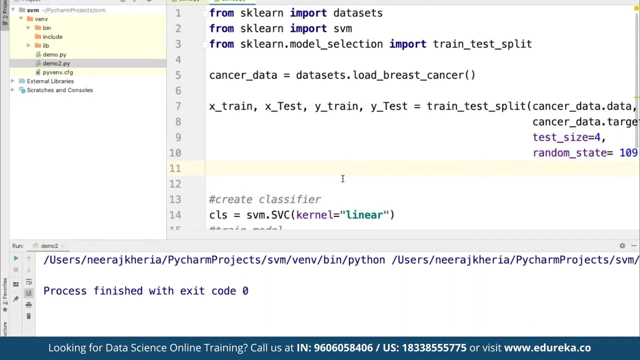 text on the x underscore test data that we already have defined. that depends upon type of data that we have. so that totally depends upon the type of all data. we are going to simply import and let's move this import from the end up here, so you have to define this in the top section from sql. we are 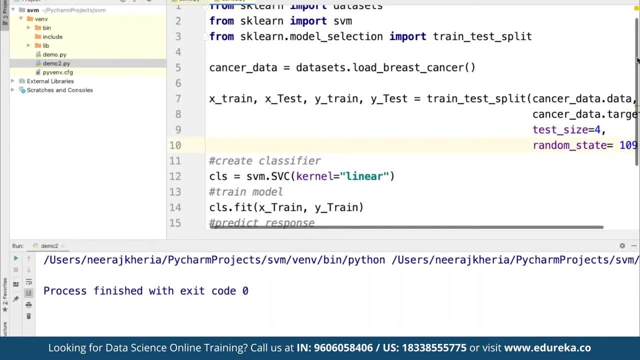 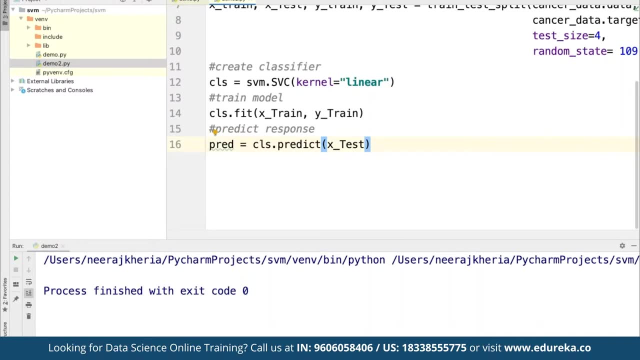 simply going to import the svm if we had to find all right, and now we have to find the classifier. now we are going to evaluate the model and for any model we can simply go ahead and define. so here from sclr we can also import other components. 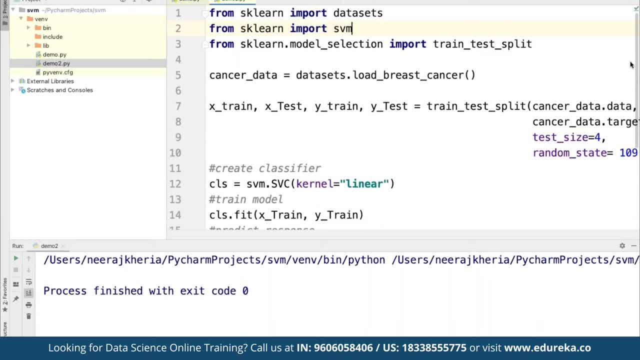 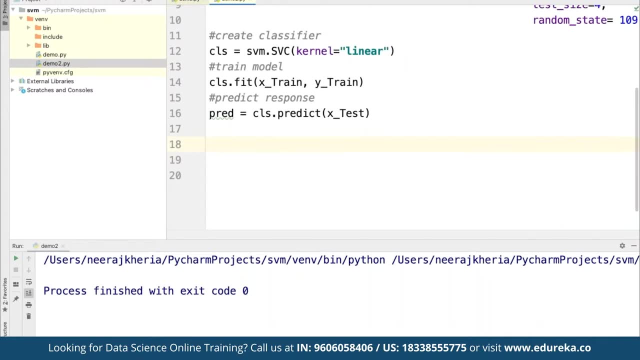 as well from sql, we are also going to import metrics. so here we are also going to import metric and by using macro accuracy metric for getting the accuracy we can define, for getting the accuracy we are going to define, we are simply going to print the accuracy of the prediction here and act for accuracy. we are simply going to define. 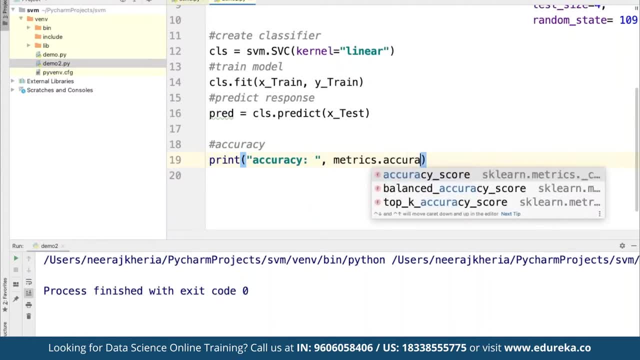 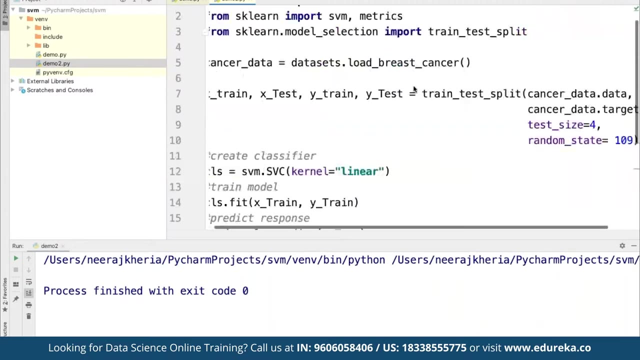 Metrics, which is again available. under the metrics that we have, we have accuracy score and then from here We are simply going to find y test and we are going to find this one for y Prediction as well, that we have defined. So I think we have used y test, we have used a park is what for? 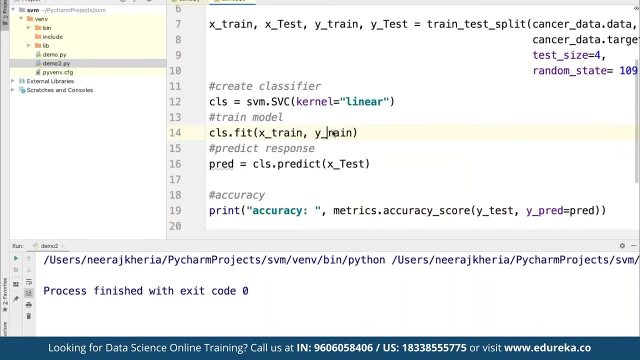 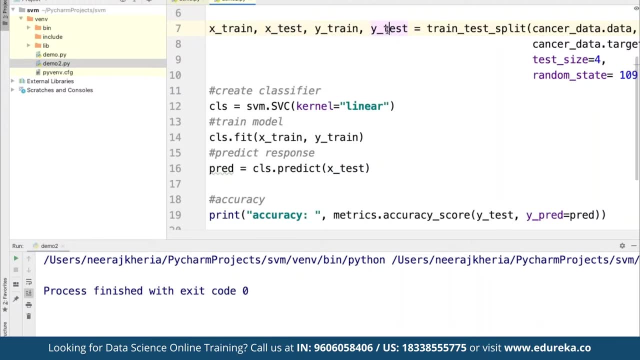 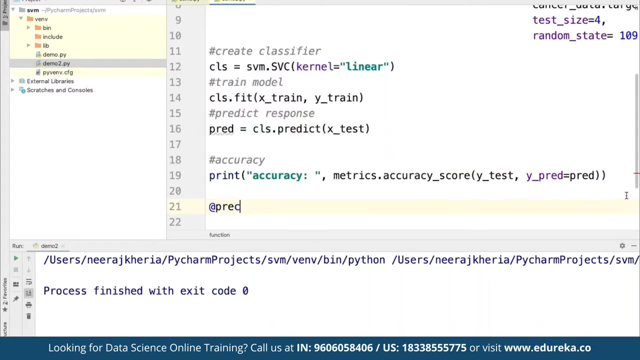 We have used less to one thing. Let's use small case for everything. just to what confusion, As it finds us test, train and test again. so you have a y test and then you depend here we define it for production and then for finding the precision score. 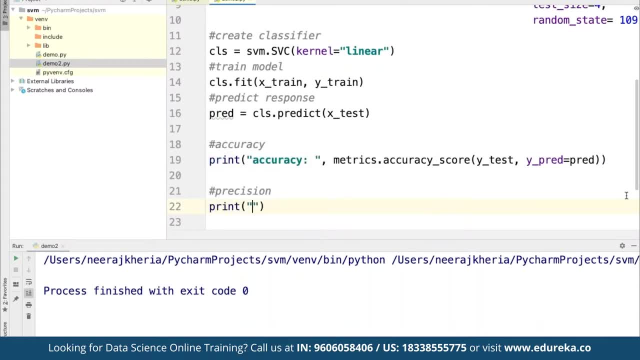 For finding precision we can simply print another statement as precision score, and In here we can again make use of metrics, and for metrics we can define the precision Score itself. So here we can define precision under score score and end here. for precision score we are going to make use of white test and 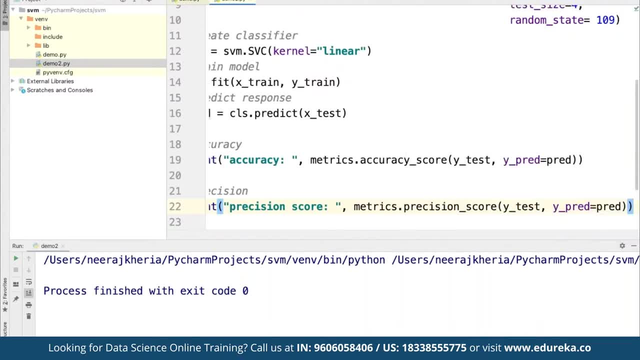 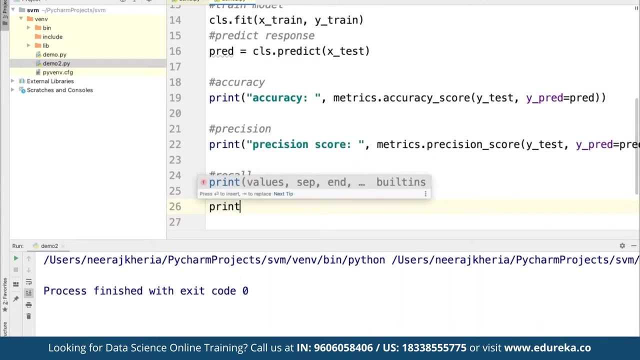 Then we are going to make use of my prediction, All right. and then at the end, if you are simply going to recall the score and we are simply going to report, So here we can define for recall, We can print under statement or recall, we get defined. 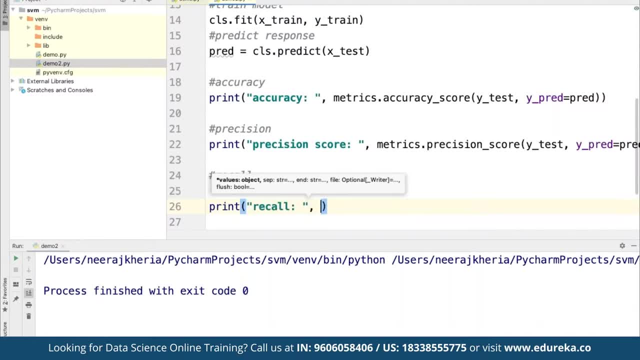 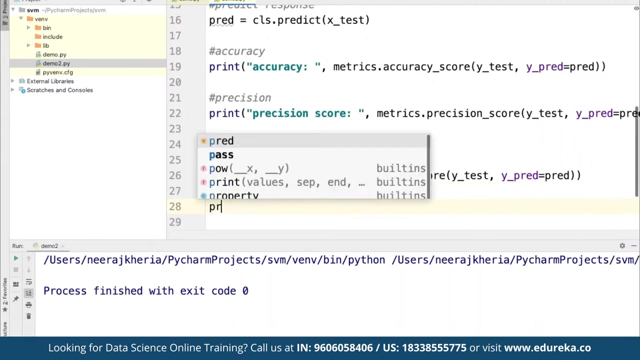 this one as recall and here from save metrics dot recall score, and for here we can define y test and y prediction for the prediction that we are going to define. and then, if you want to print all the metrics, so here we can define print metrics dot classification report, and for that we are going to make use of y, test and y.